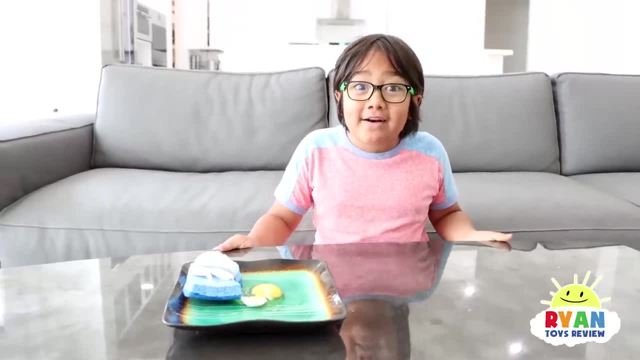 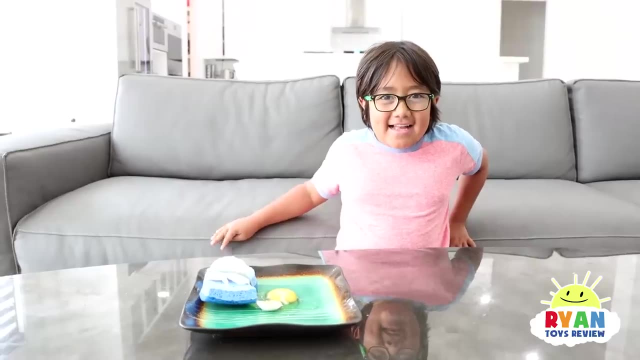 Don't give up Pombo. Together, we're going to learn how to save an egg from breaking Combo Bunga, And we can each do our own experiment and then come back together with our own results. Okay, let's go. 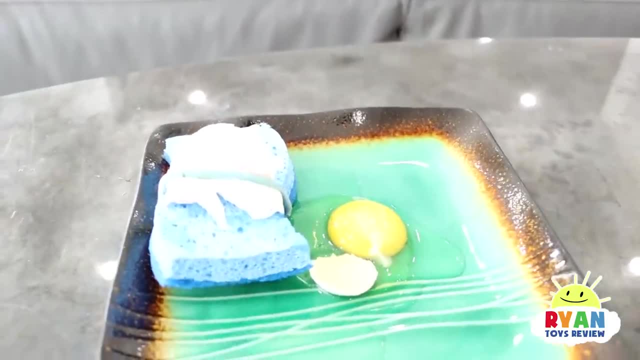 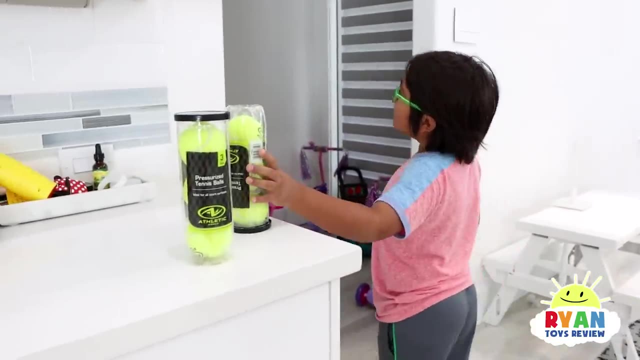 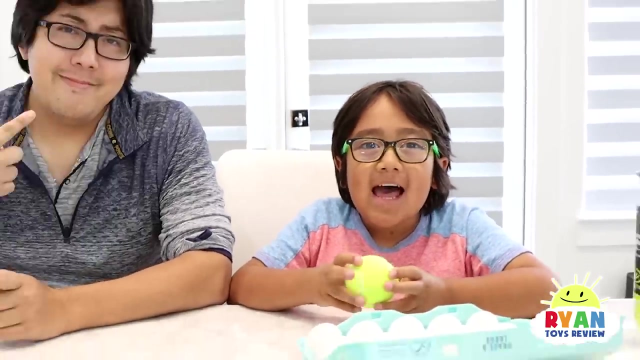 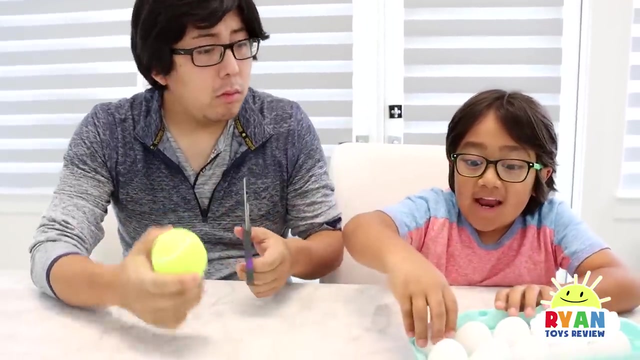 What could save an egg from being broken? Tennis balls. Remember always to ask a grown-up for help, Which is me. Alright, let me see. What do you want me to do, Ryan? So Daddy's going to cut open the tennis ball and then we're going to put an egg inside and see. 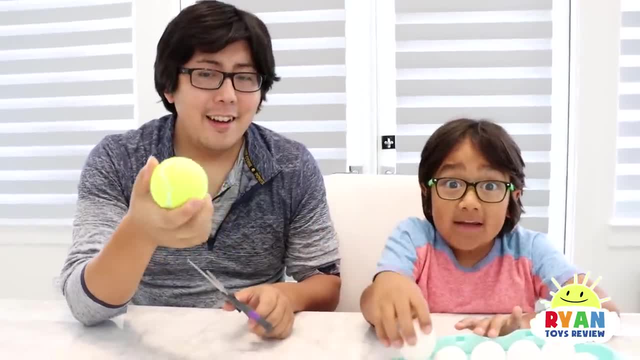 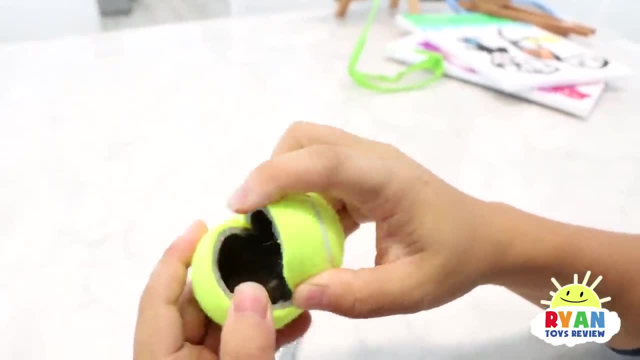 if the tennis ball helps it from breaking. Cutting a tennis ball is very difficult, so always ask a grown up for help. I think we got it. Look, Wow, that's what it looks like the inside of a tennis ball. It kind of looks like a Pac-Man. 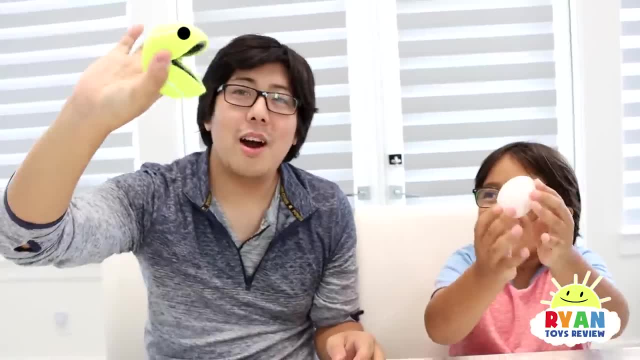 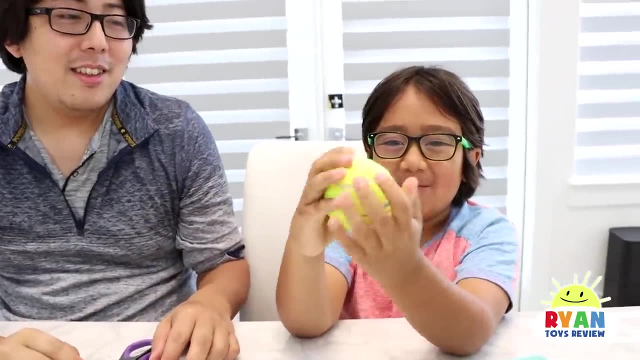 Daddy, Walk-a-walk-a-walk-a-walk-a-walk-a-walk-a Walk-a-walk-a-walk-a-walk-a-walk. Do it, Daddy. He's eating the egg. Ah, it fits perfect. 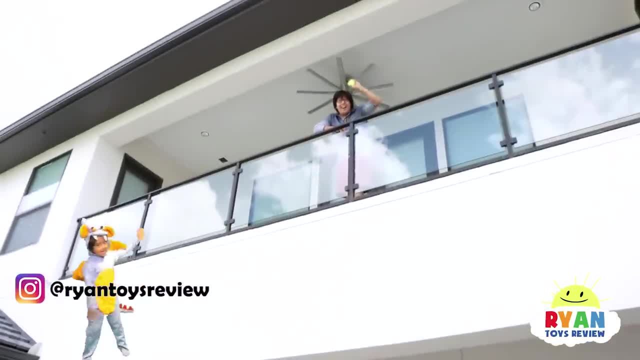 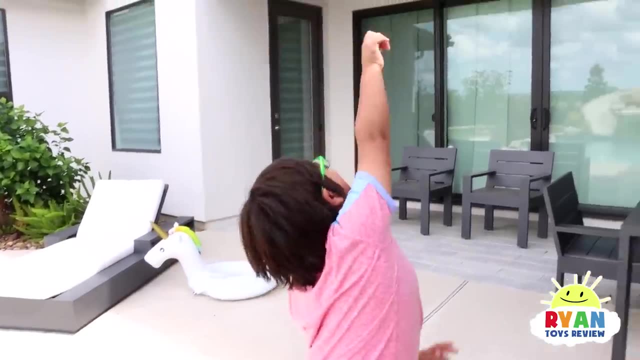 Okay, guys, Hey guys. Daddy's all the way up there, Hey guys, And he's gonna drop the tennis ball to see if the egg breaks. Go Daddy. All right, here it is the tennis ball with egg inside, You see it. 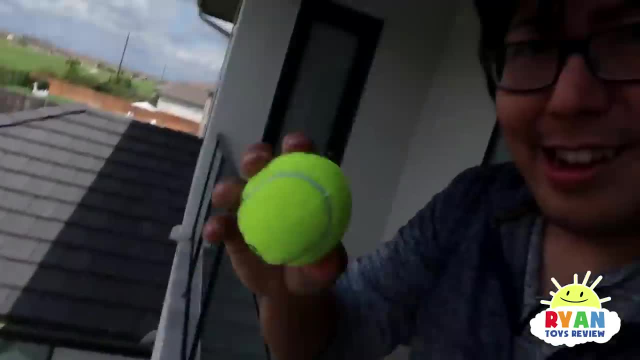 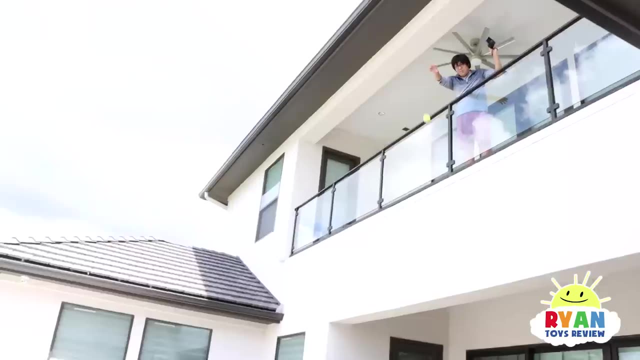 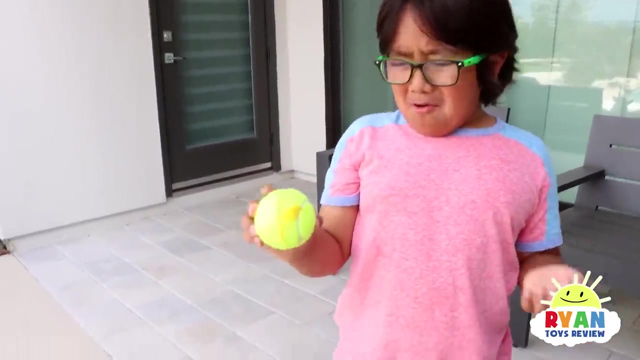 And Ryan's down there waiting You ready, Ryan. Yeah, Here we go, guys, Let's see what happens. Three, two, one go Go Guys. look It didn't work. The egg is definitely broken. 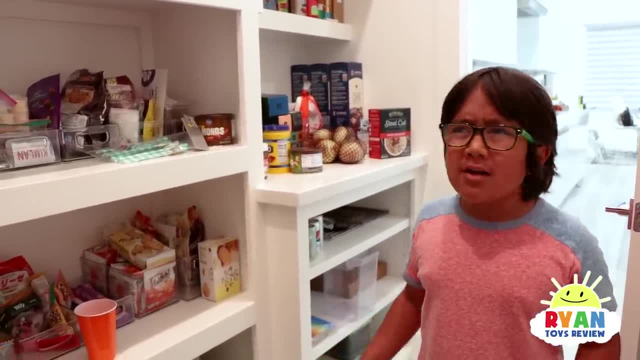 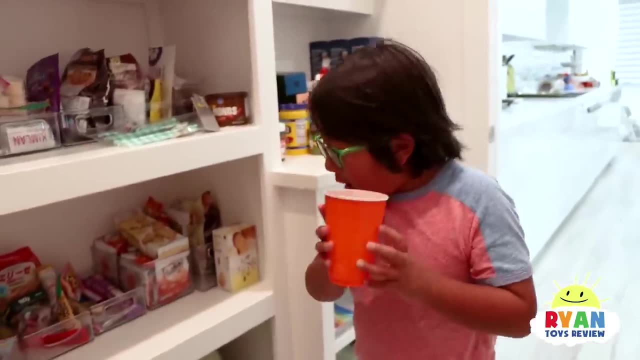 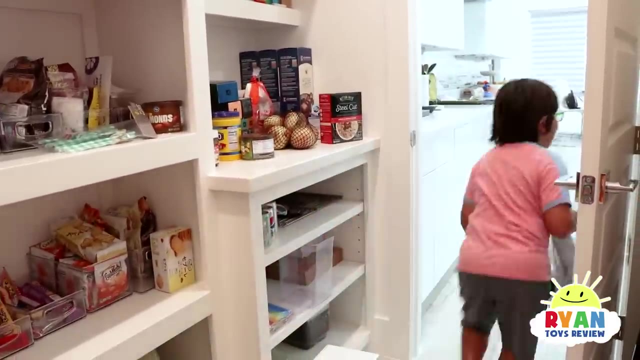 That one didn't work. I wonder what else there is. I have an idea: We can use a cup and a bag to make a parachute. Let's go Yay, Now Daddy's gonna help me make a parachute for the egg. 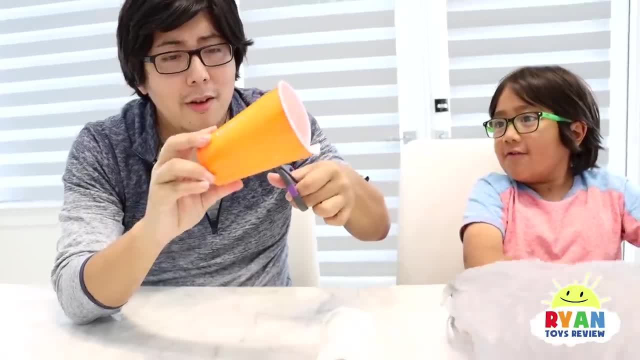 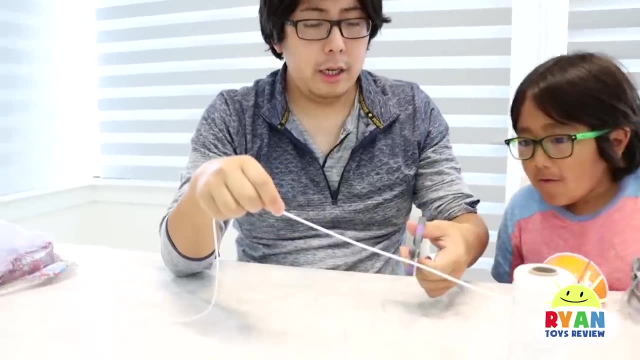 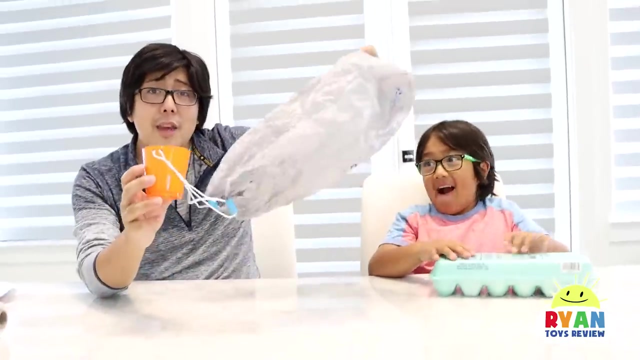 Yeah, I'm cutting up the cup right now so we can make a place for egg to go in, And you need some strings. I'm already a parachute, Whoa, And after you put them together, it looks like this: Boom. 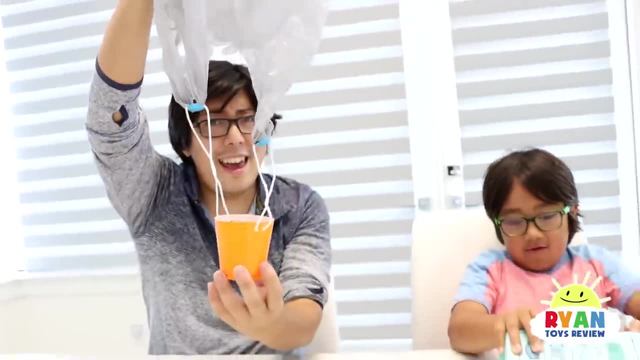 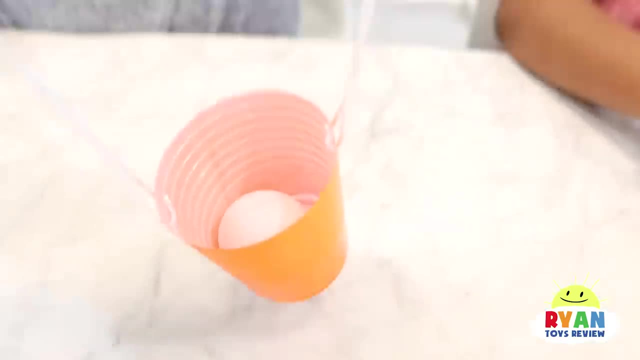 This is a parachute and this is the pocket that carries the egg. All right, put it in, Ryan, Let's see if it works. Boom Whoa. Oh yeah, it fits perfect. I think it's gonna work. All right, let's test it out. 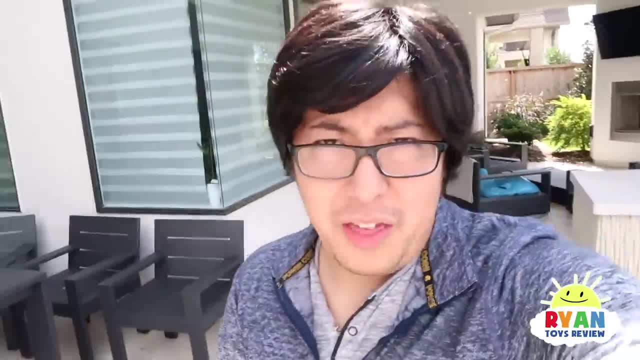 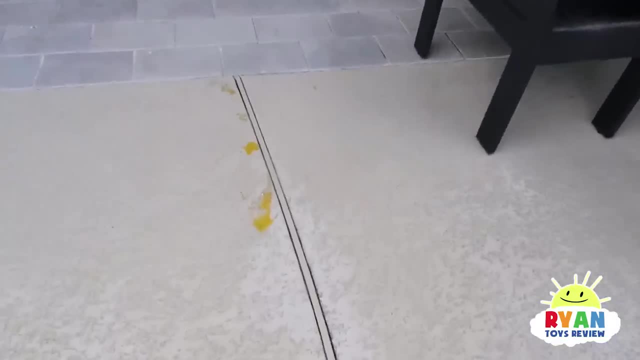 So I'm outside waiting for Ryan to toss out the parachute with egg. Let's see if it's gonna work. Hey, Ryan, Hi, Hopefully it works because, look, It's harder to clean. Look, Look at this big mess. 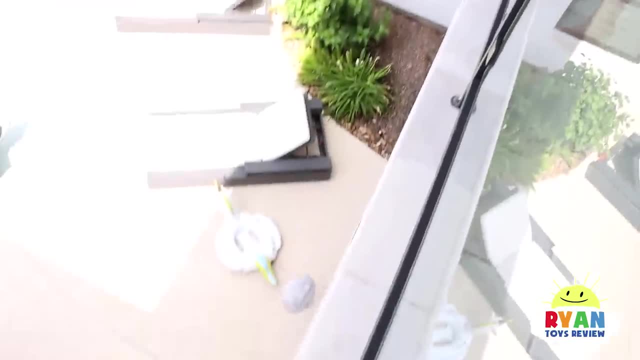 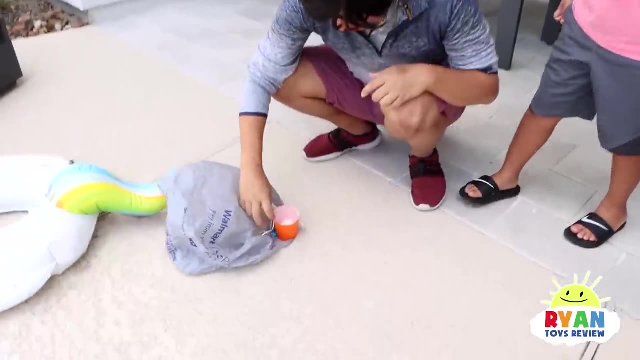 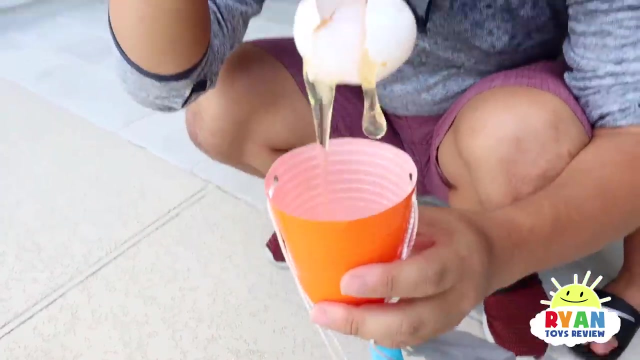 Three, two, one. All right, let's see. Daddy, did it work. Oh no, it didn't Look at this. Oh Aw, Uh-oh See, All right, it's okay, We can try the next one. 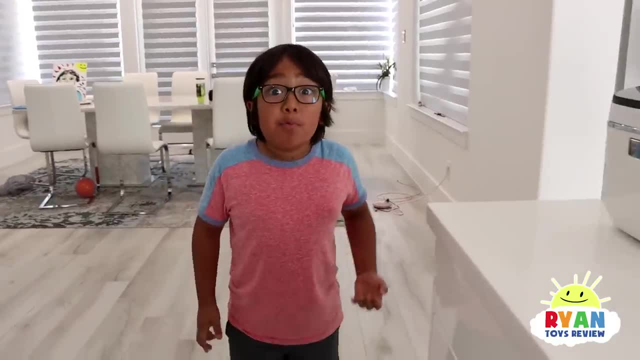 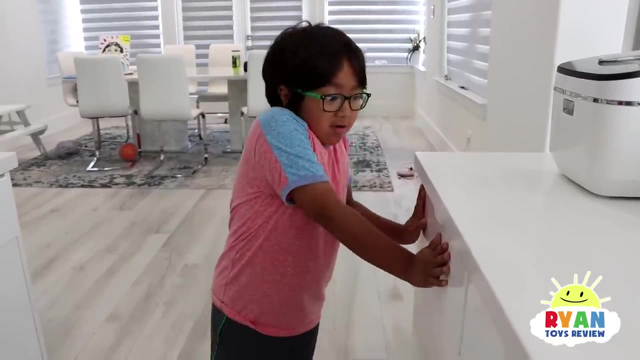 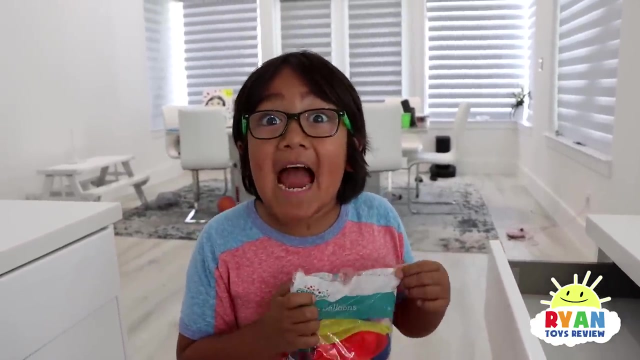 Yeah, let's do it. Aw, So far both of my ideas didn't work. Hmm, I wonder where I could get another thing, Maybe in here: Balloons. Maybe we can use balloons to help the egg from breaking. 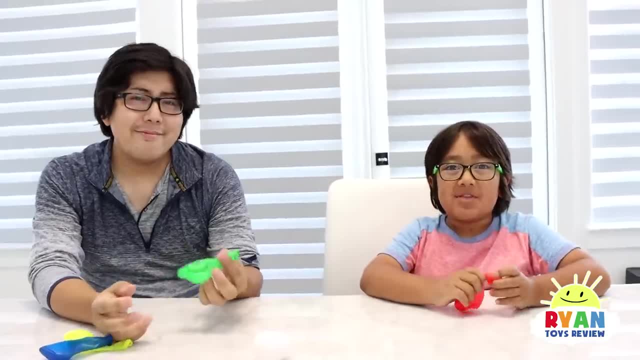 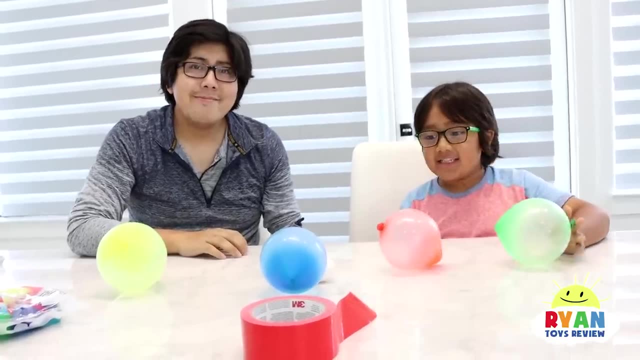 Let's go Now. let's blow up some balloons. Yeah, just like small, like that. Yeah, perfect size. Next Daddy's gonna wrap all the balloons around the egg. All right, let's see. Okay, Make sure you cover. 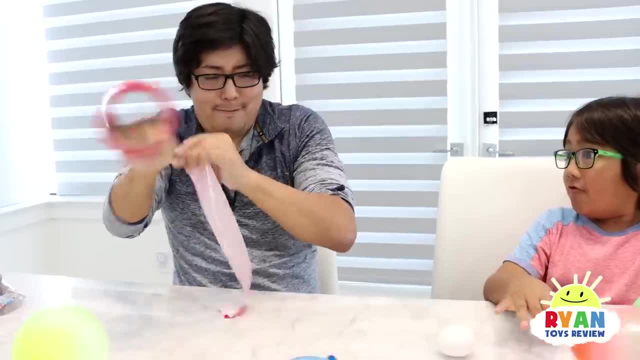 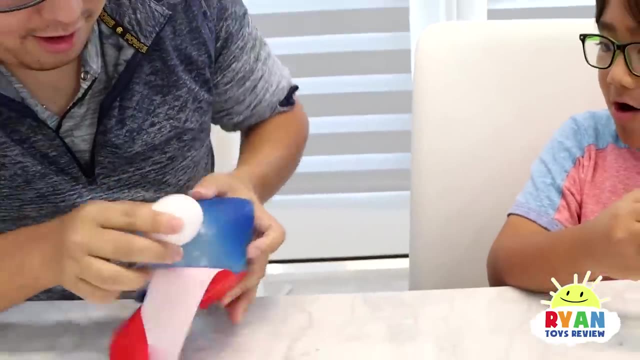 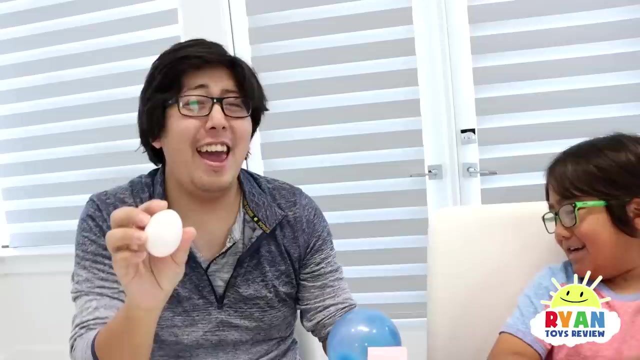 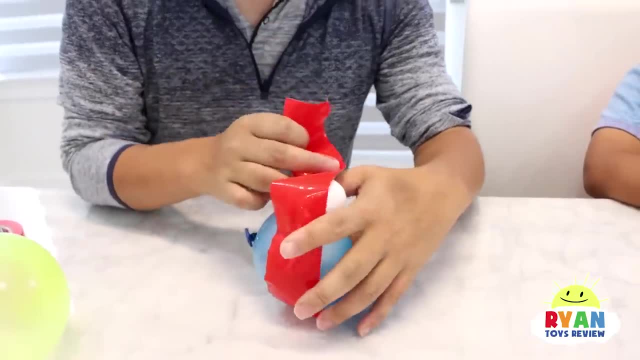 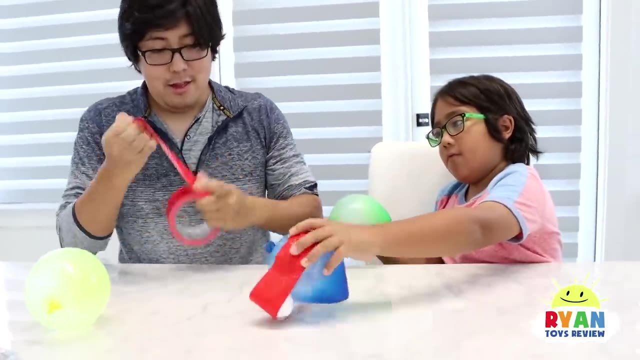 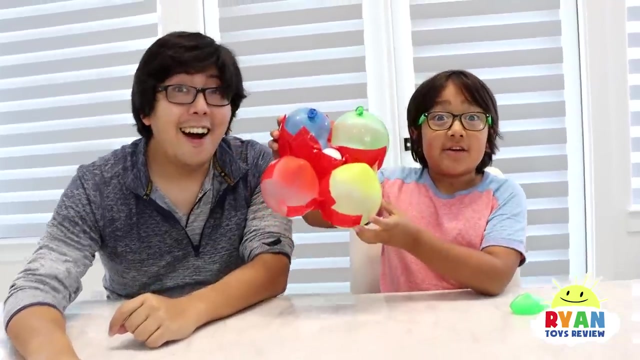 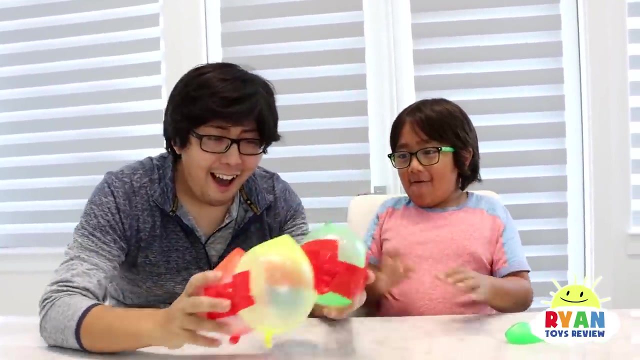 Okay, I'm sorry, I guess accident happens. Mmm. Yes, Secure, Good, All right, Give me the next balloon. Okay. Okay, This is a good start, but now let's put more balloons. All right, next time we need a bigger balloon. 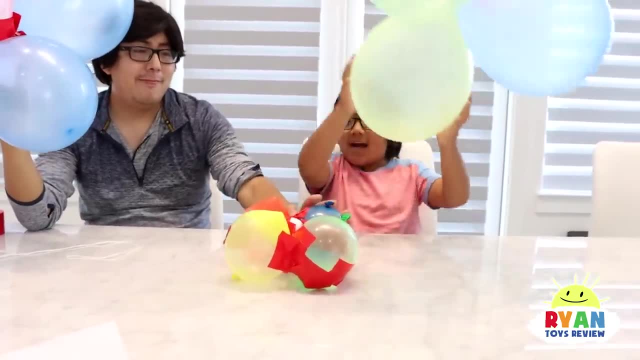 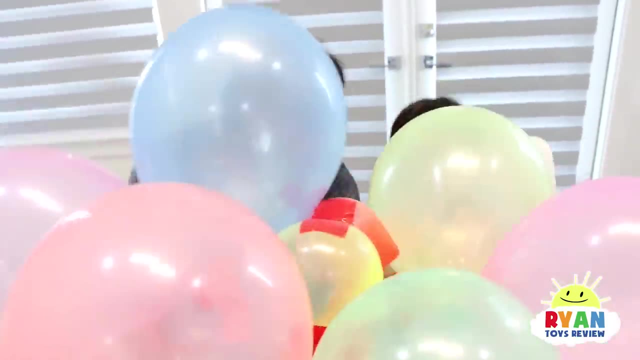 Now we have big balloons. We're gonna take this side to this side of the egg and we're gonna take the other one to this side. Ah, Looks like it's gonna work, Ryan. Yeah, Whoa, And this time we're done. 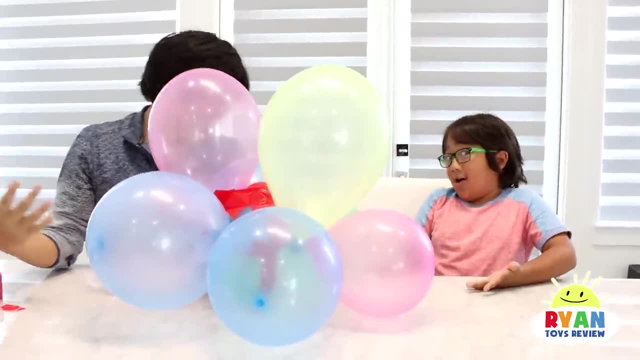 Woo-hoo, Looking good, I think it's gonna work. Yeah, All right, let's go upstairs and test it out. Ooh, Woo, Okay, guys, I'm on the balcony. I'm ready to test it out. 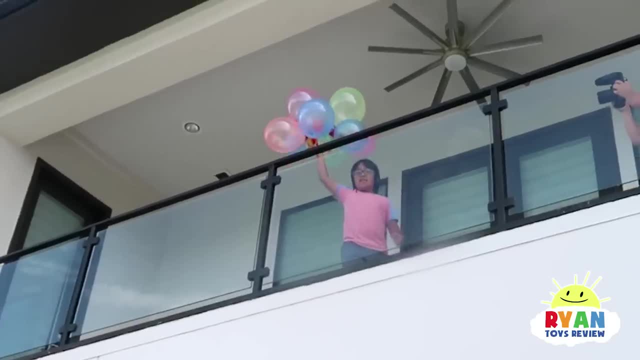 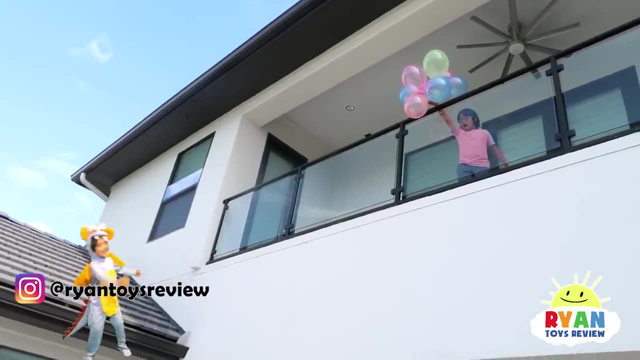 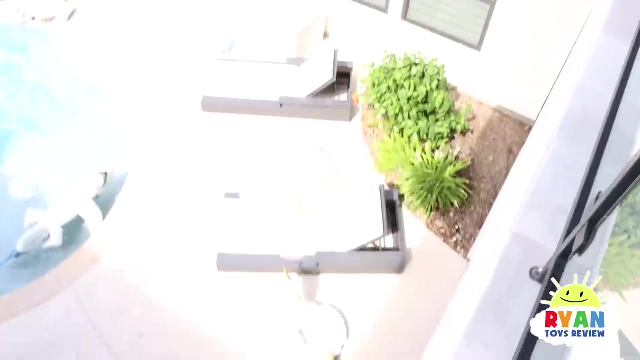 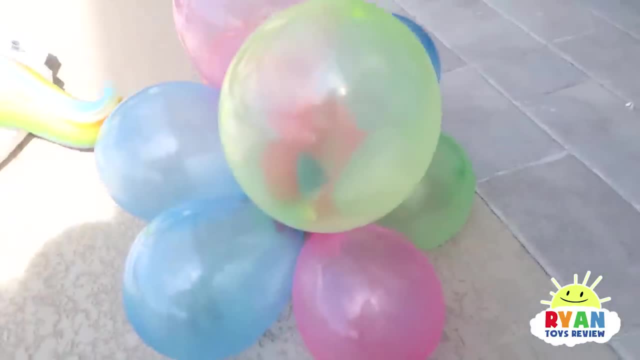 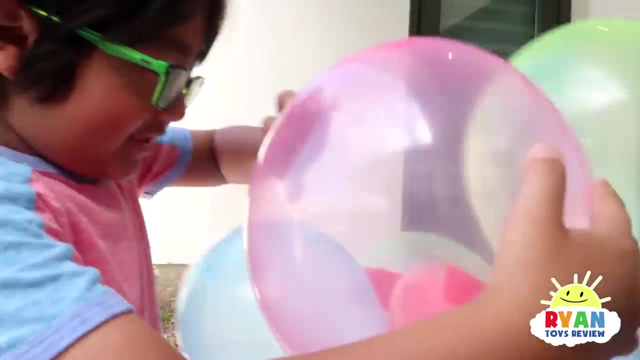 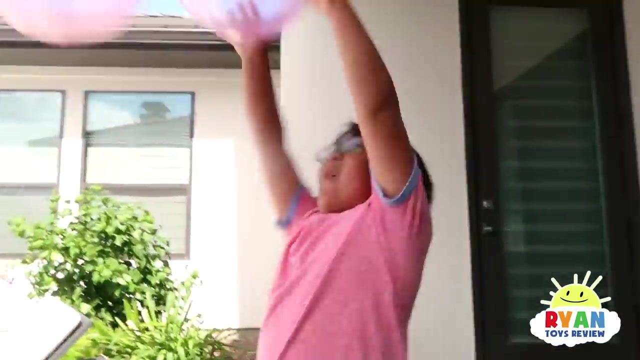 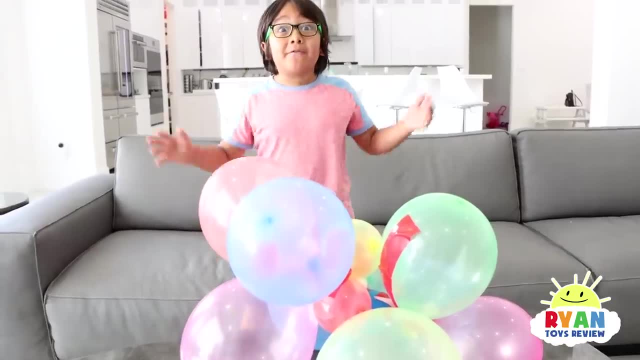 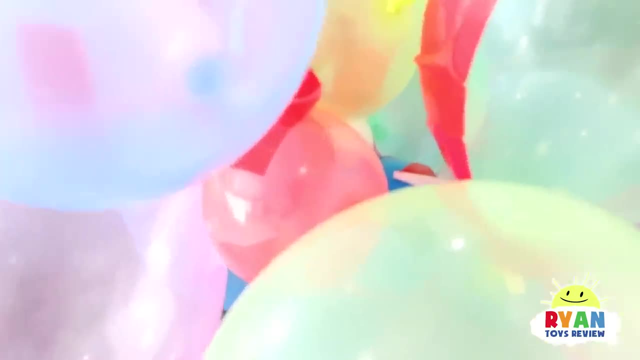 It didn't break. Whoa, we did it. guys. Let me see Whoa Pombo To work. But just to make sure, let's open it up. Look, Combo, it worked. The balloon saved the egg from breaking. 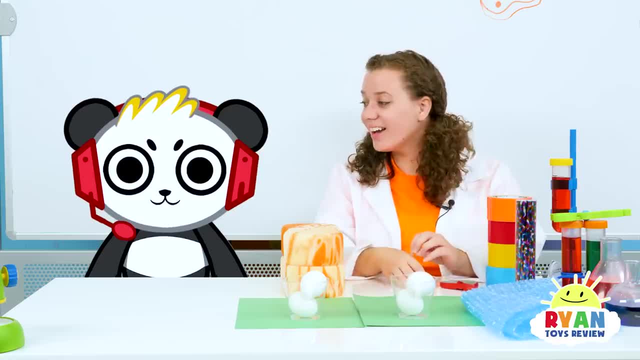 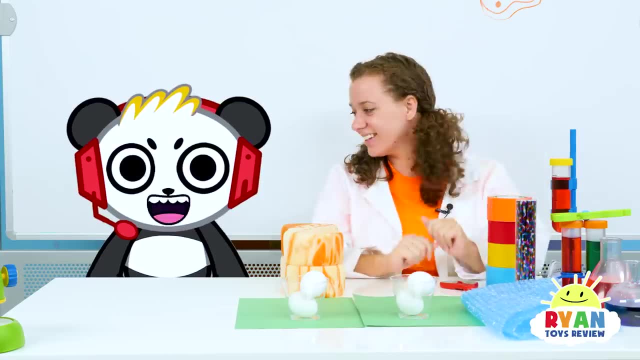 Did you get yours to work? Okay, Combo crew. now it's time for me to do my experiment, And I got my assistant Bree here. Hey guys, Make sure to always get adult supervision when you're doing these experiments. 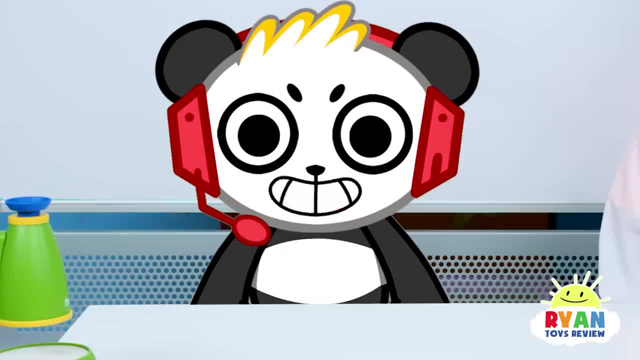 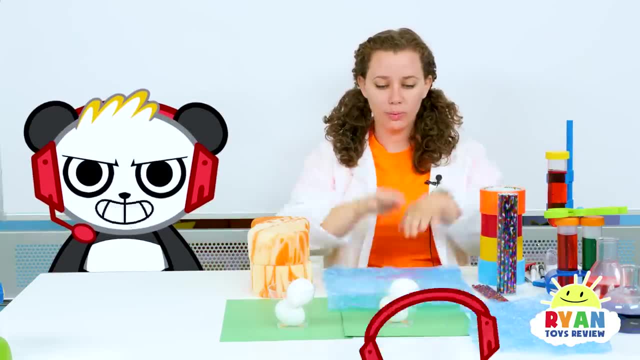 All right, so first up is egg plus bubble wrap. Egg plus bubble wrap equals safe egg. All my headsets that I order online come wrapped in bubble wrap And they're always perfect, So I think they're going to do a great job at protecting these eggs. 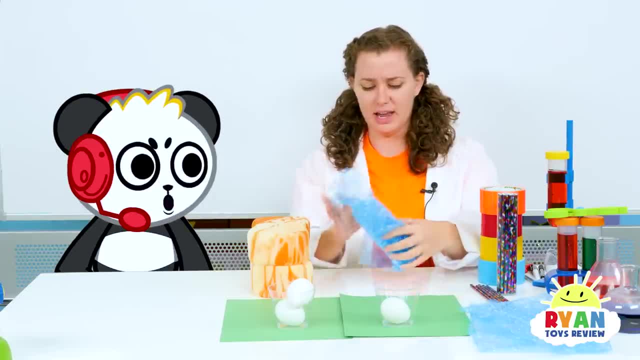 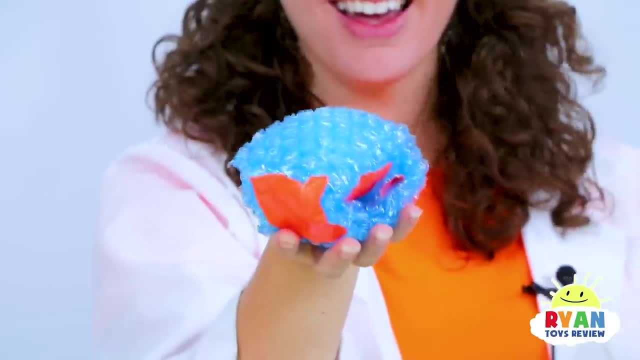 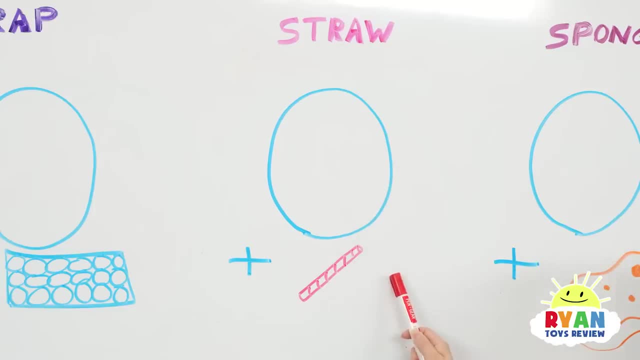 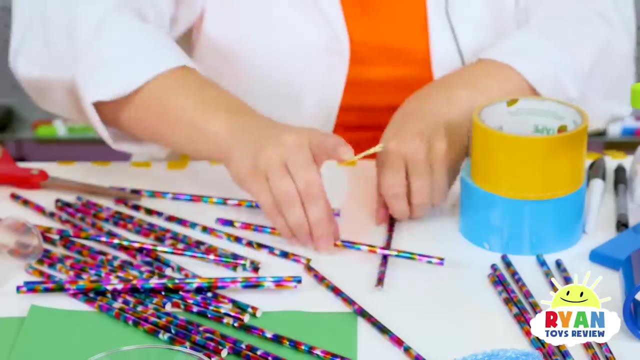 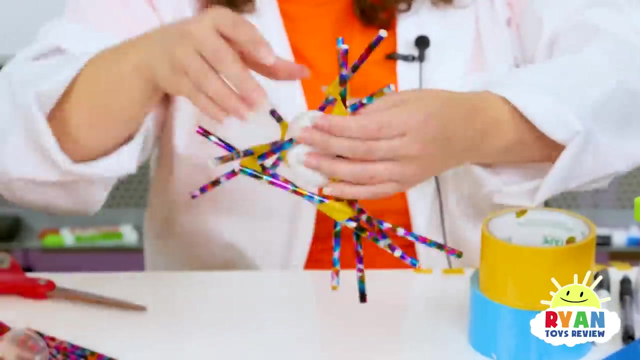 Yay, And now it's egg plus straws. We've got our nice straws there, all colorful, cutting up our duct tape. Then we tape our straws together to make like a nice egg protecting machine. So it should protect the eggs perfectly. 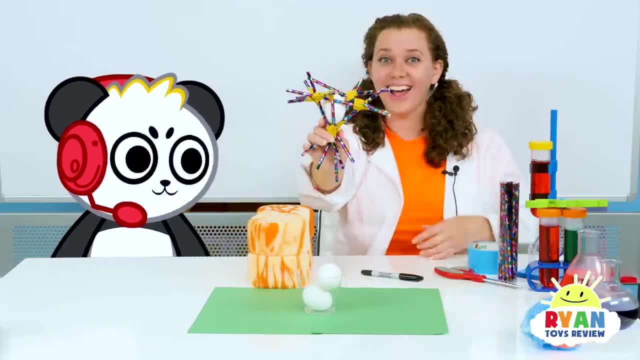 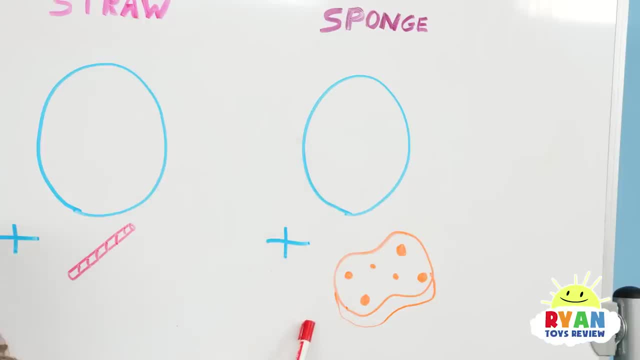 Whoa, check that out, Combo Bunga. that looks so cool, But I wonder if it'll work. I guess let's move on to the next one. And last we have egg plus sponges. First we got to open the egg. 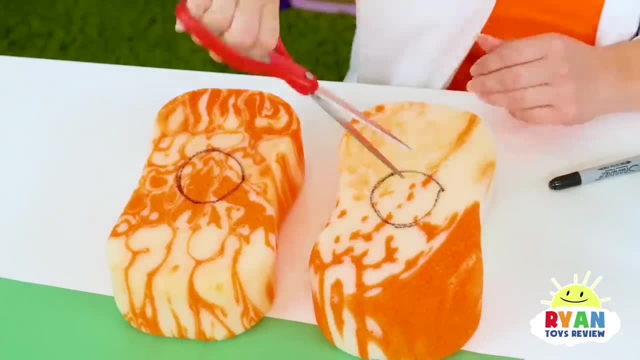 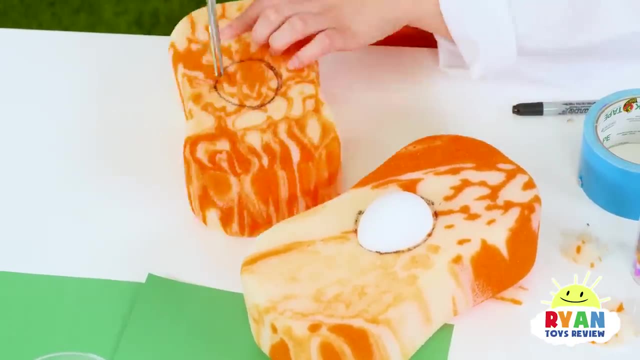 And we're going to outline where we're going to put our egg. And then we take the scissors And be careful as you cut a hole for your egg. Okay, we got one down, Now let's get the other one. Hopefully, I think these two can work together to protect this egg. 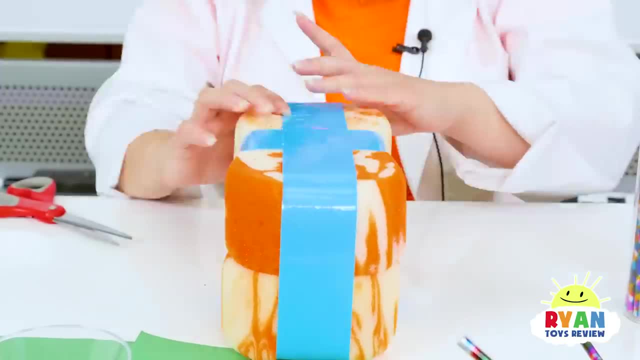 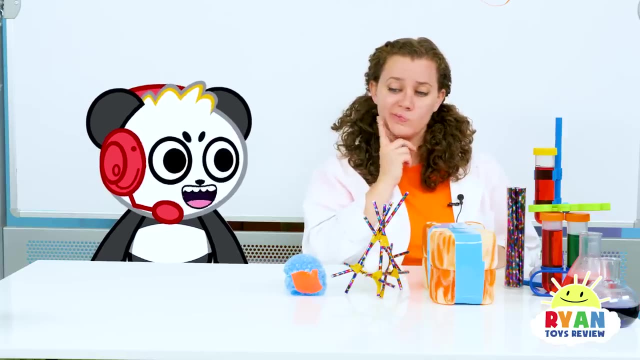 Hey, we got an egg sponge sandwich. The sponge sandwich looks really cool. Which one do you think is going to work- though My money is on the bubble wrap, I think it's going to work. I think it's going to be the sponge. 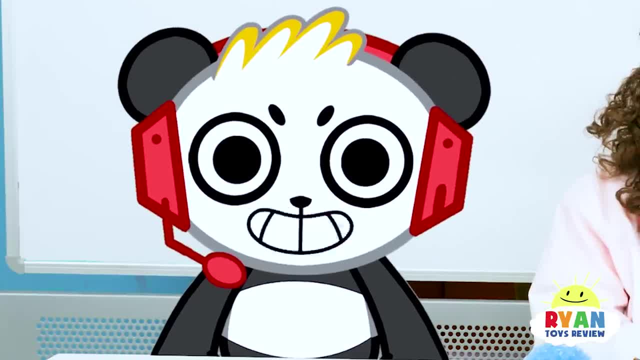 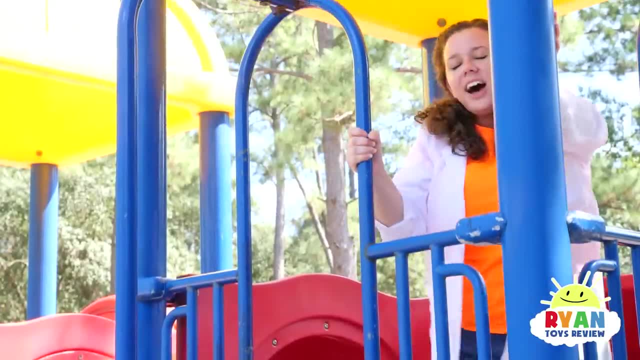 This has the most cushion around it. Well, there's only one way to find out To the park. Let's do it. Whee, All right, Hey everyone, We made it to the park. Combo, are you ready for the drop? 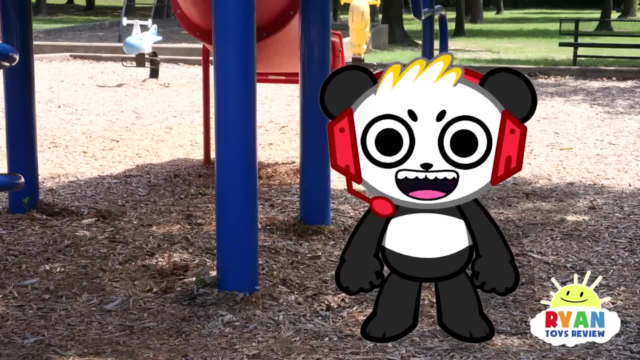 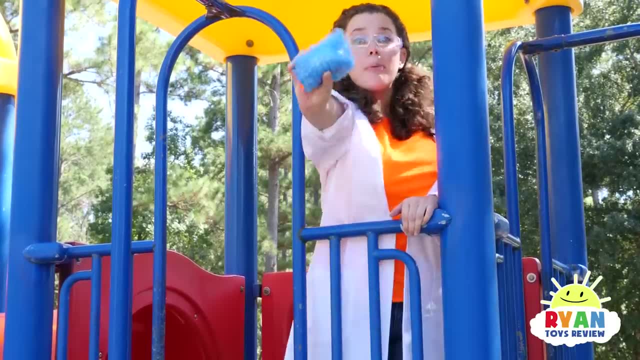 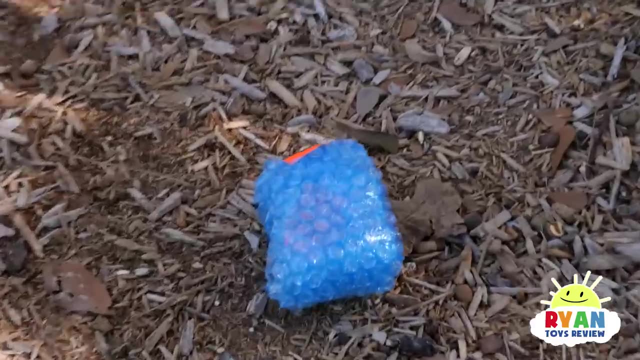 I'm so ready. Now, Bree, let's start with the bubble wrap. Oh, but first safety goggles. All right, First up is the bubble wrap. Yeah, let's go. Three, two, one, All right. 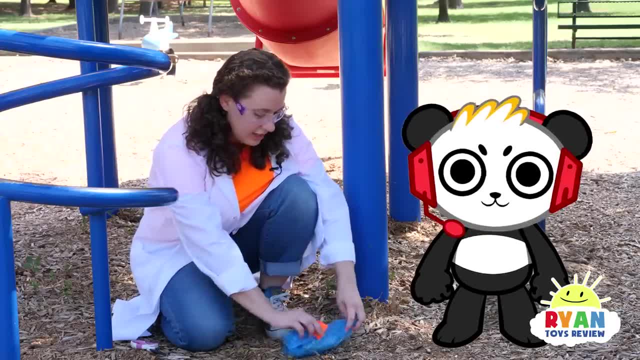 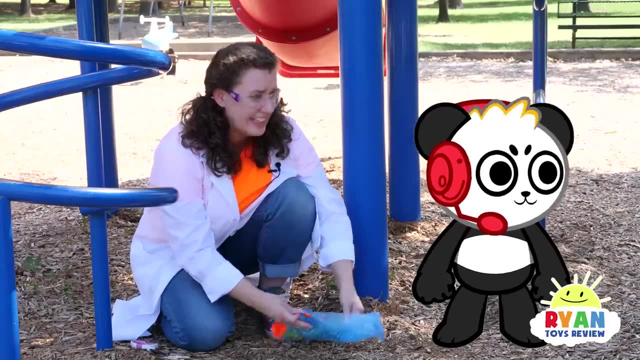 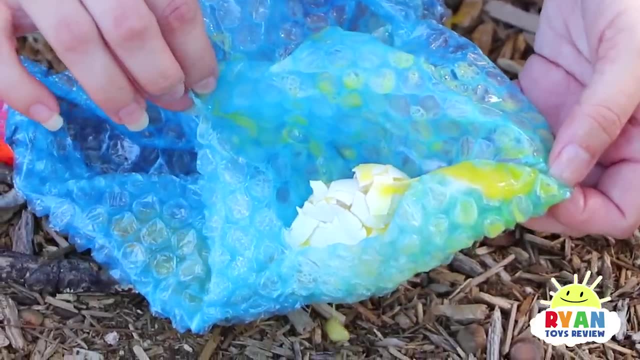 Let's check out this egg. Okay, let's see Combo. I'm not sure your guess did so well, It feels a little flat. Oh no, Oh, it's not looking so good. Oh, Maggie, It's all broken up and stuff. 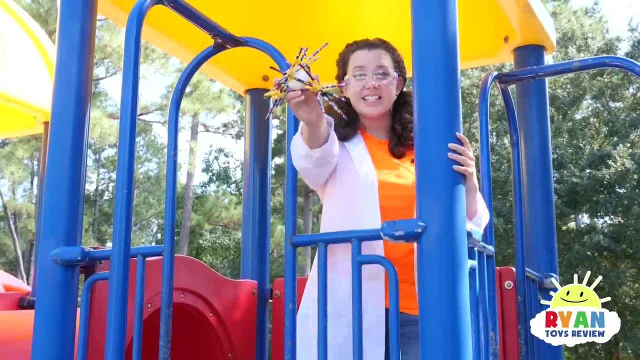 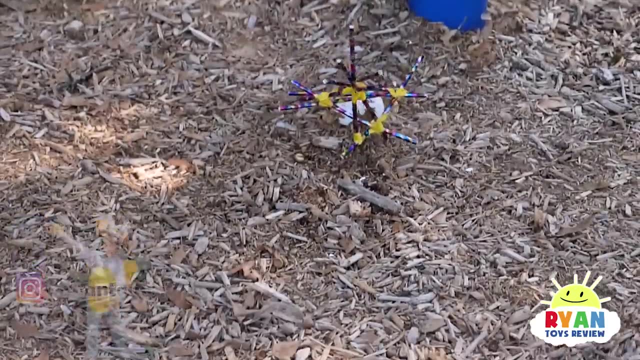 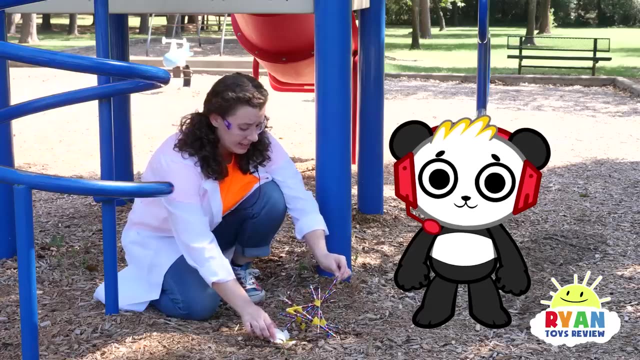 On to the next one. Okay, here comes the sticks in three, two, one Slow motion fall land. Whoa, did you see that It exploded? Yeah, it's not looking so good, Combo. I don't think this one made it. 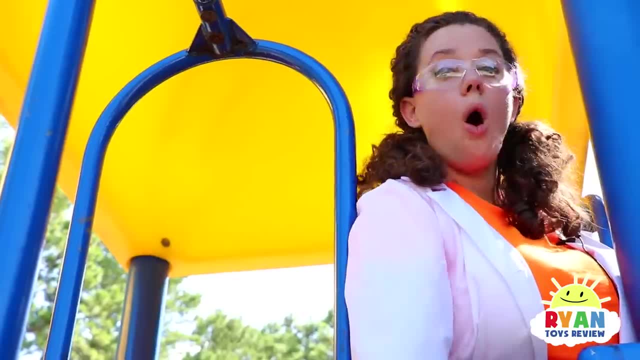 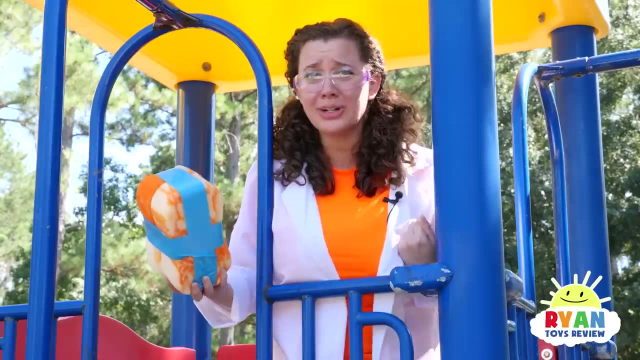 Well, I just hope the next one works out better. Moving on to the sponge, So this is our last one and it's my guess It has to work. It's orange, I'm orange. What could go wrong? Are you ready, Combo? 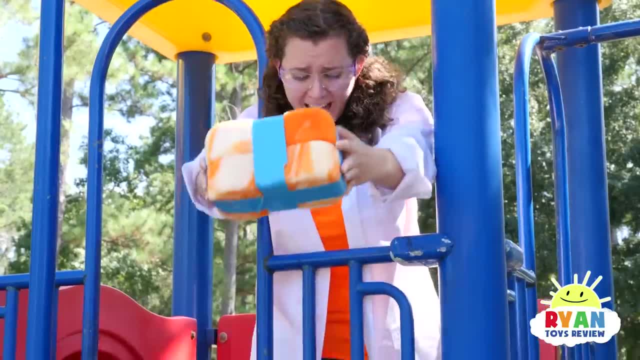 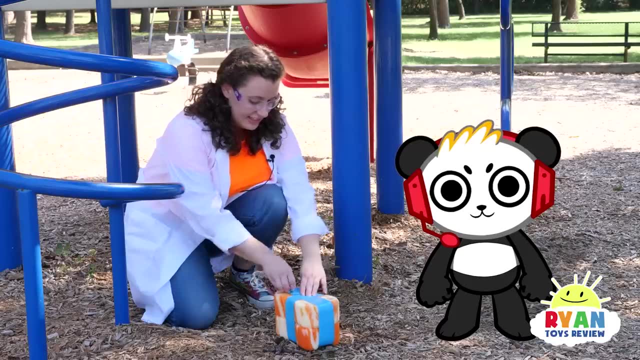 Toss that sponge. All right, three, two, one, Three, two, one. Whoa, I saw it bounce. It sounds really good. Let's see how it did. Combo. All right, let's see Whoa. 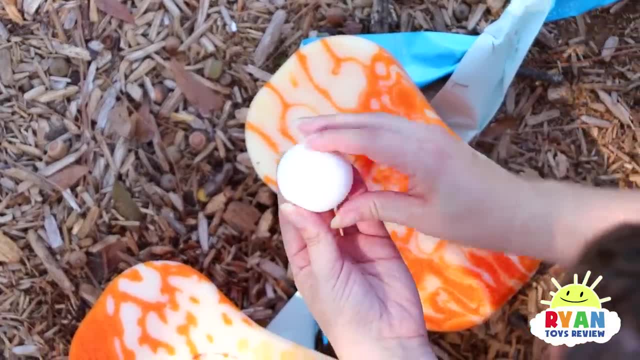 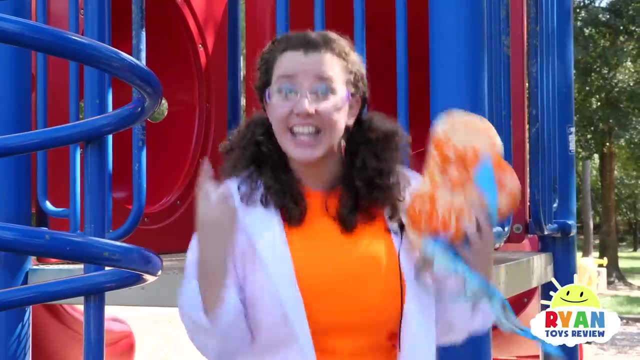 Wow, it worked. Combo- Look at that Way to go. Eggie- Yay, we saved Eggie. Okay, so we got our results. Now let's go to the lab and take a look. Let's go, Let's go. 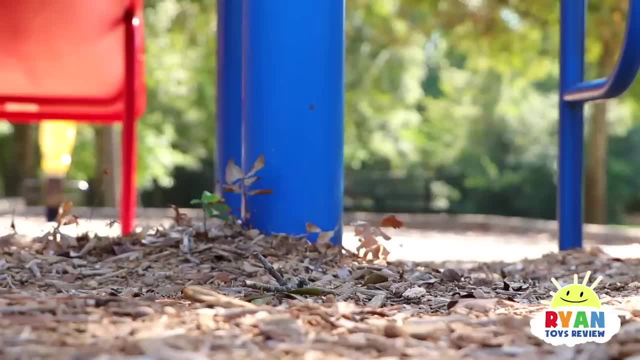 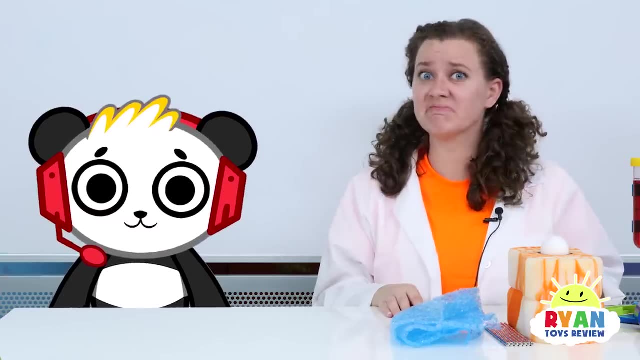 Let's go First up. we had the bubble wrap. Now it looked like it worked really well, but when we opened it up it broke into a whole bunch of pieces. Yeah, that one got really messy. That's a no. 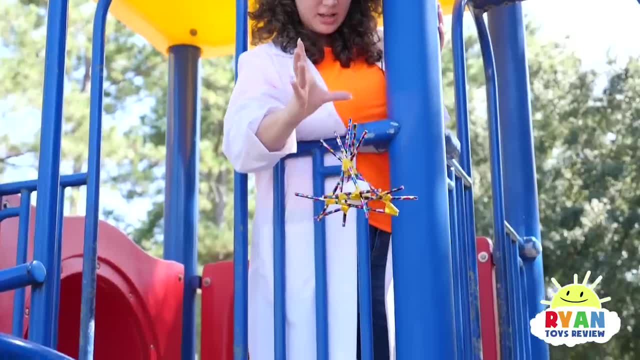 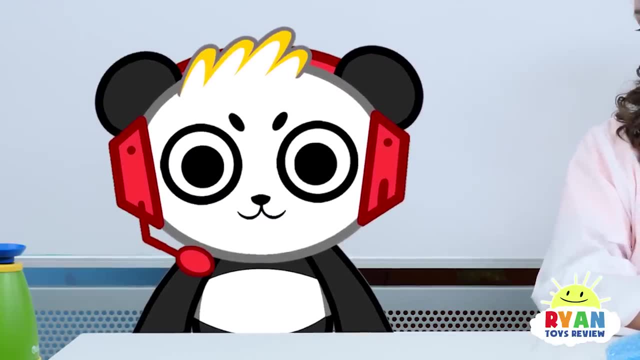 Ooh, then we had straws. Now, when this dropped, we could tell it didn't work at all. Yeah, that one was super messy. It's a no from me. Well, the last one was my guess. Not saying I'm right, Combo, but I was right. 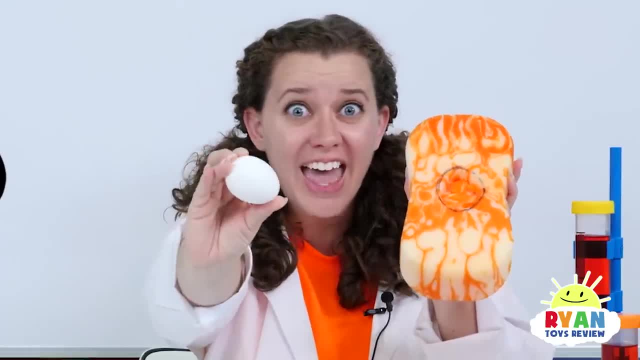 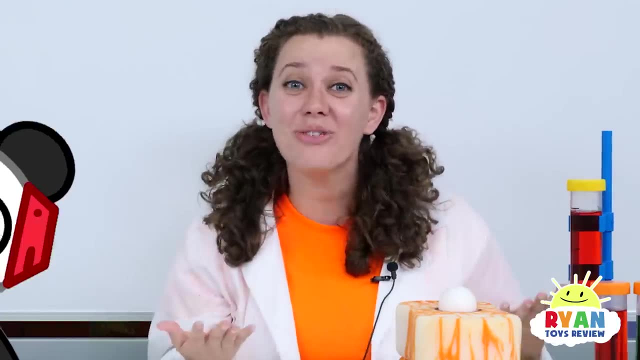 It was the sponges. And look, They worked so good. we still have the egg. All right, he sure is the winner. This was a great experiment, wasn't it Bree? It really was. It was so much fun. 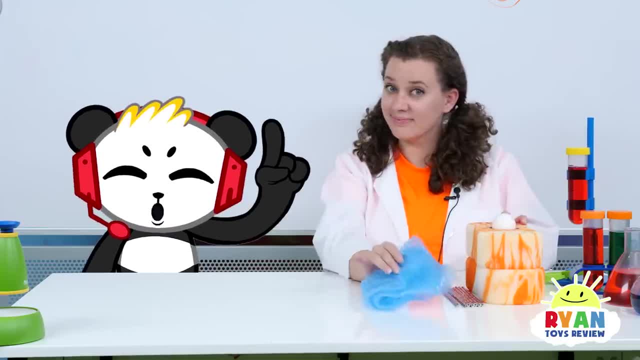 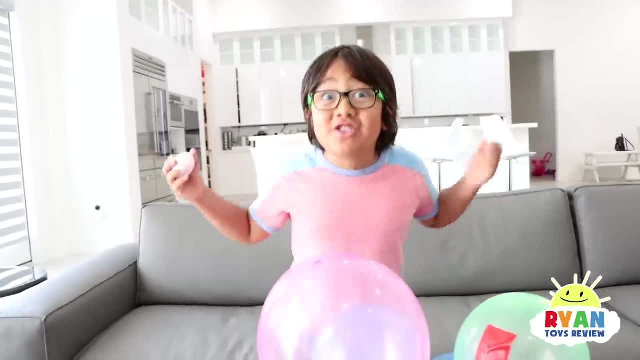 Combo Crew. remember that we did this experiment with a bunch of household items, so you can do this too if you want to, But make sure you got parent supervision. Yeah, that's so cool. I had so much fun doing an experiment with you, Combo. 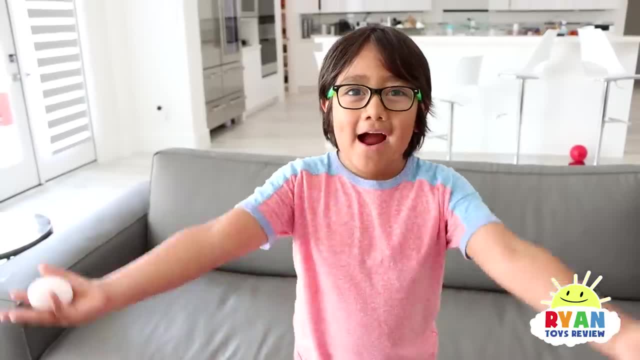 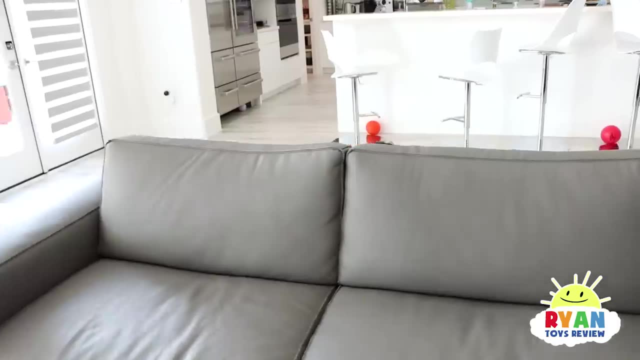 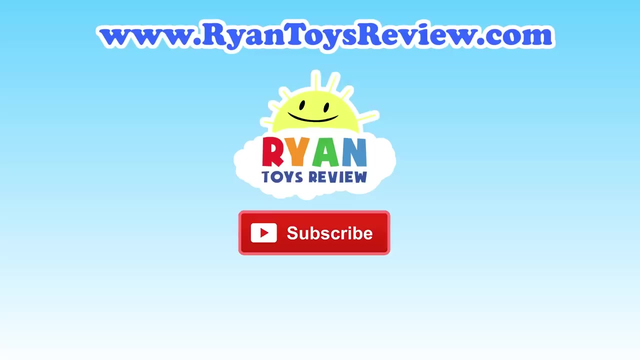 Bye, Remember always stay happy and rise up. Bye, I'm okay, Rise up. Please click on one of these videos for Ryan Toy Room and more fun. See you next time, Bye, Bye.